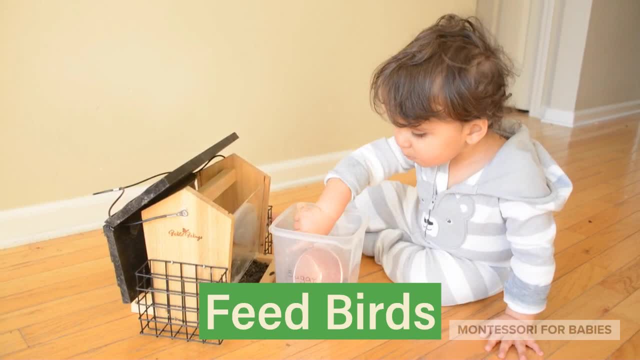 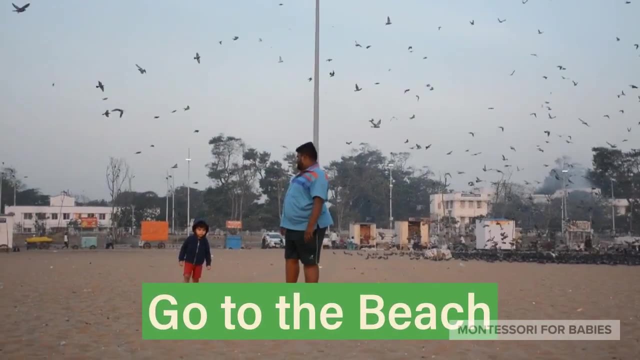 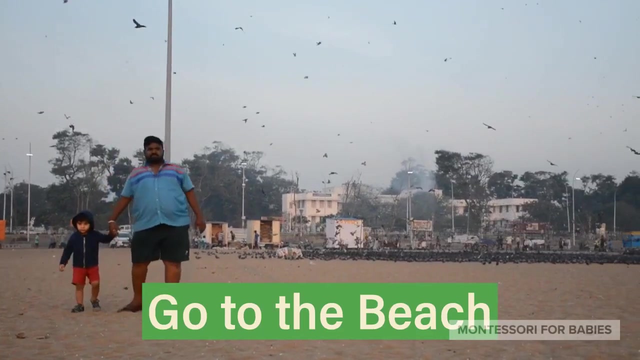 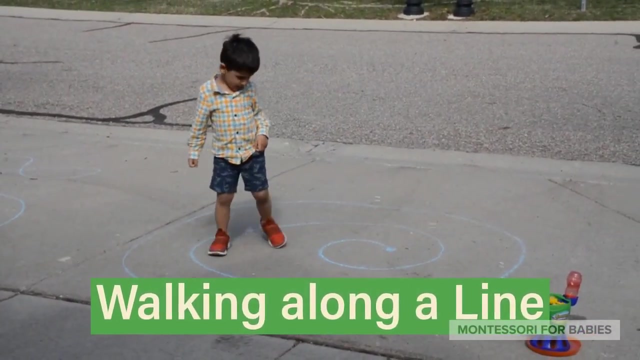 the bird feeder at least once a week to keep the seeds and the birds safe and healthy. Visit the beach, maybe with buckets, shovels, sieves, a floating boat toy, a dump truck and maybe even a picnic lunch that your child can help set up. Invite your baby or toddler to walk along lines. 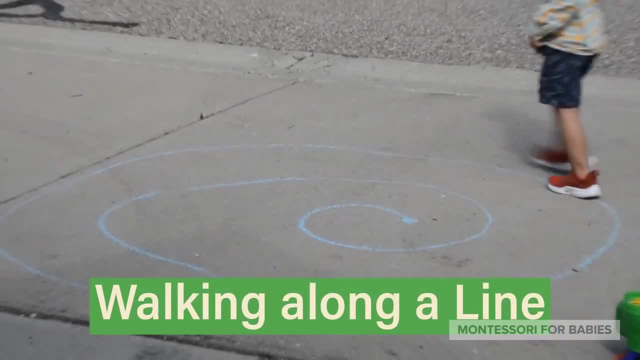 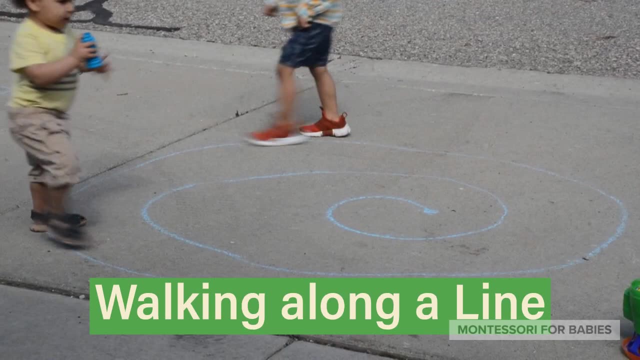 that you find or make yourself Walking on lines outside can be used as an informal precursor to the more structured walk the line activities that older toddlers do in the Montessori classroom, where they learn to walk perfectly straight, foot after foot, sometimes balancing a bell. 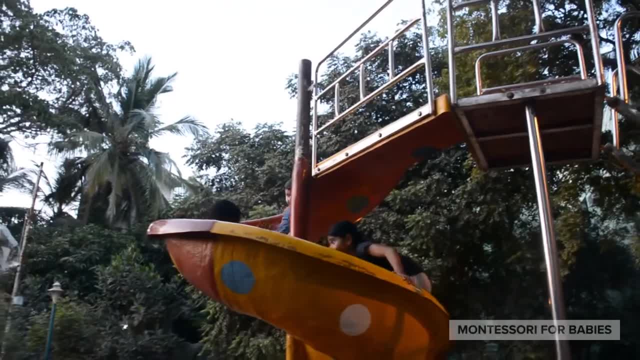 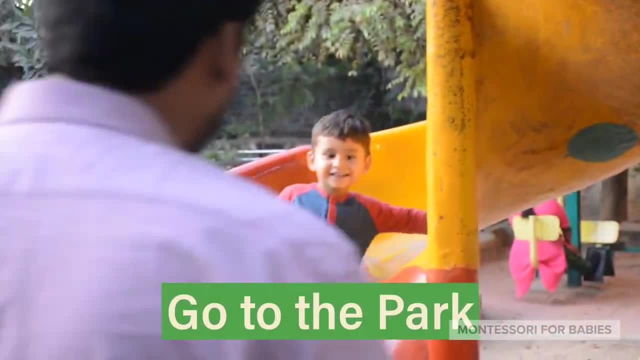 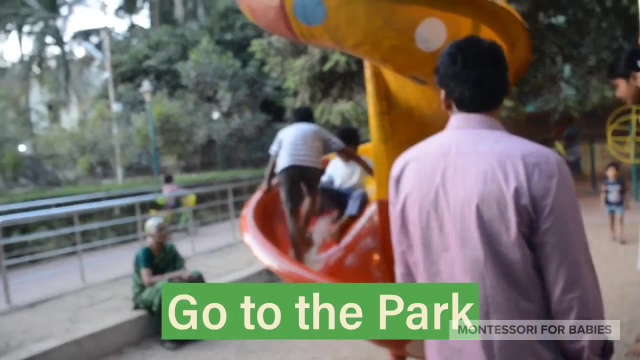 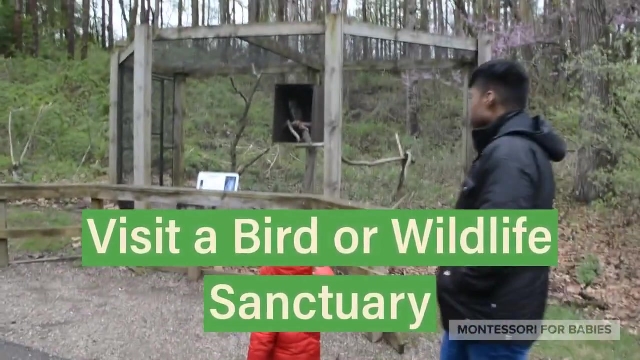 or objects on a spoon along a line on the ground. Go to the park. Playground equipment offers many opportunities to practice postural control, balance and coordination, upper and lower strength and social skills. Visit a wildlife or bird sanctuary, While you can also visit a zoo. 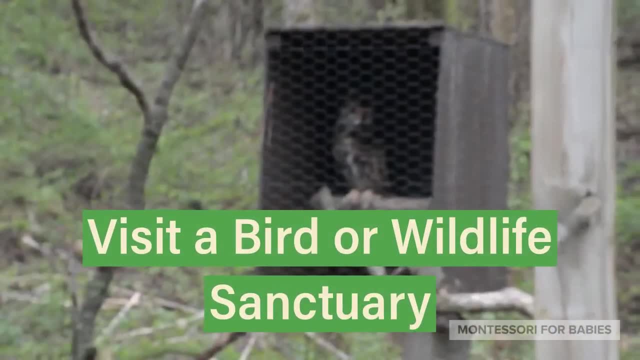 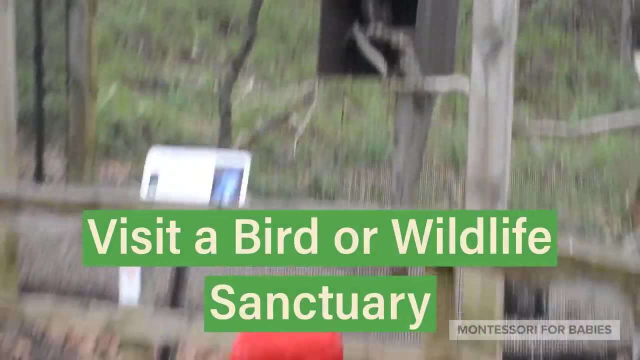 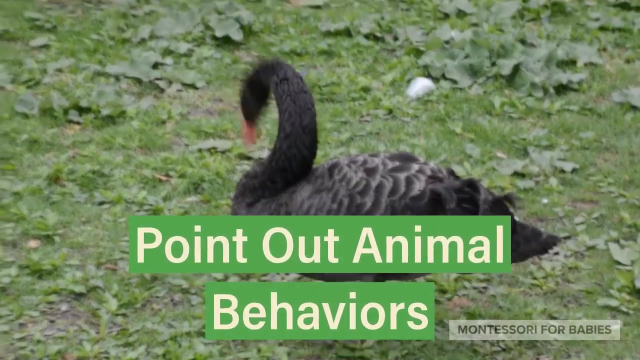 these sanctuaries often allow children to see local wildlife in their native habitats and focus on native local conservation. They are also more affordable, less crowded and less overstimulating than zoos. if that's a concern for your family, One thing you can do anywhere as point. 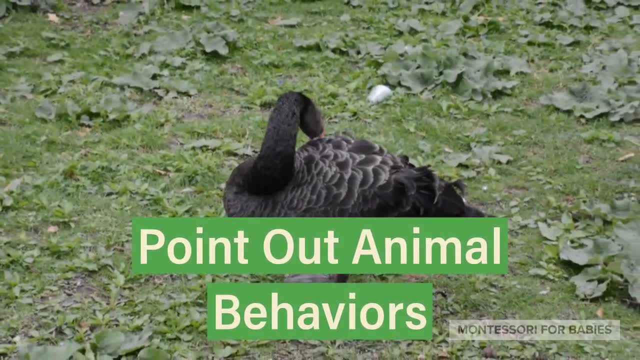 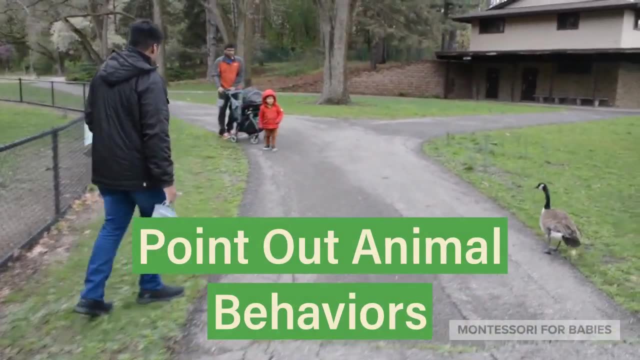 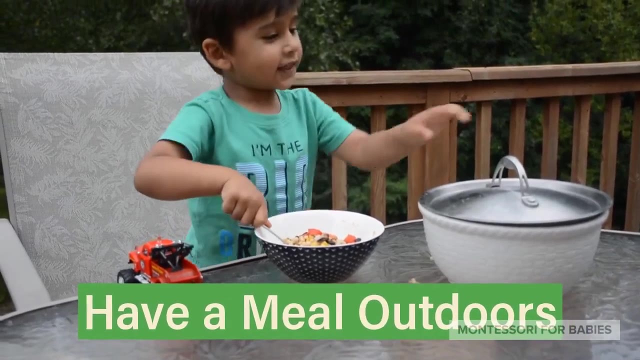 out animal behaviors. Learning about these behaviors and imitating them is fun for children and, if done in a respectful way, can instill a sense of respect for animals, as children learn that these animals have lives of their own, Do regular activities outdoors, like having a meal. 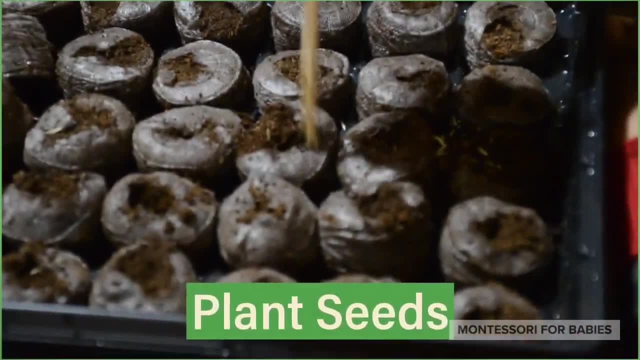 plant seeds and watch them grow. Peas, sunflowers and pumpkins are big and easy for toddler fingers to handle. Marigold and perennials are still available in the wild, but they come in different varieties. They are often great for your child and your family. Some animals are believed to be. 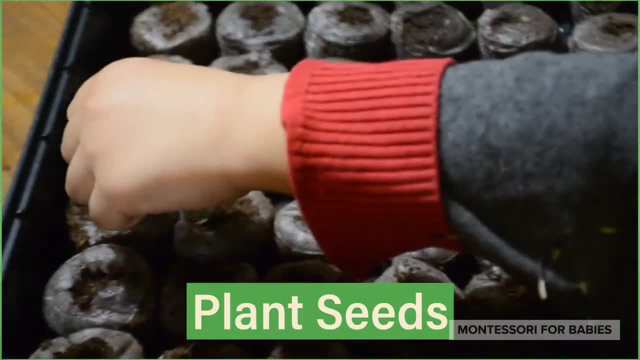 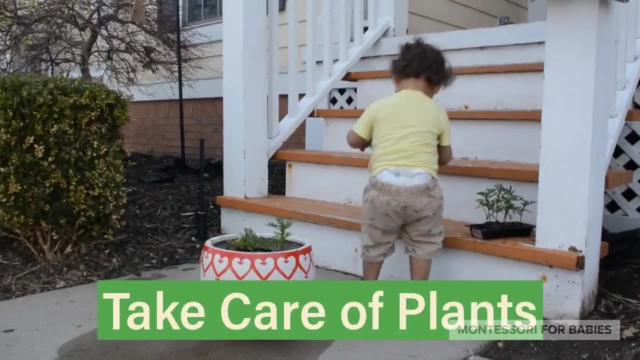 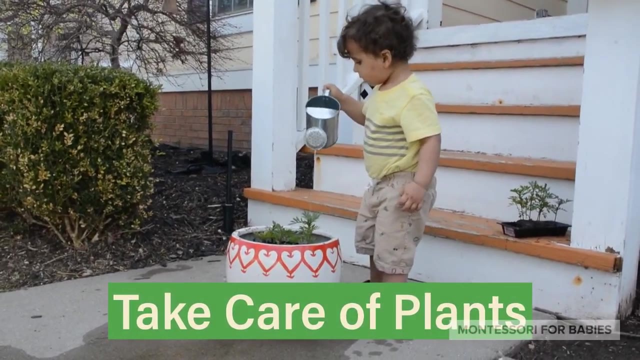 Marigolds, radishes and cornflowers are fast growing, but the seeds are smaller and harder to handle. Invite your children to take care of plants. These can be your plants grown from seed or ones that you buy. Care can include weeding, watering, pruning, composting or harvesting.